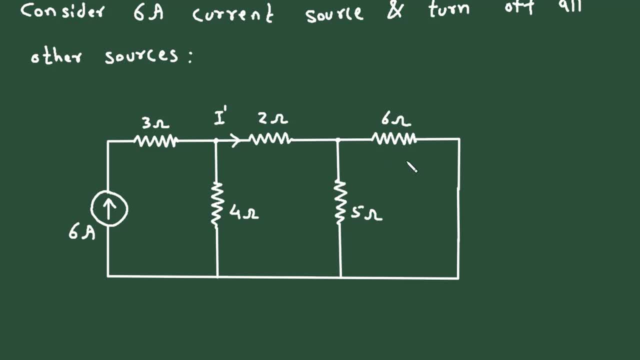 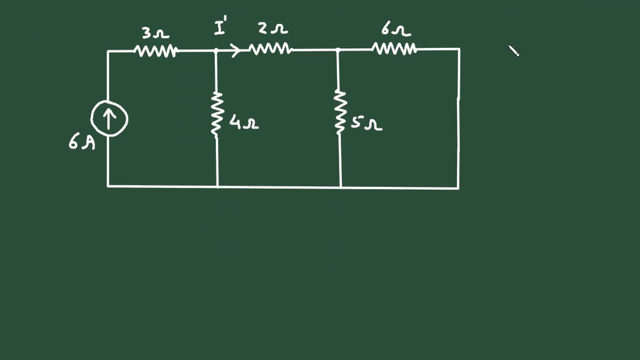 Now, as we can see here, this 6 ampere and 5 ohm, This 6 ohm, 6 ohm and 5 ohm are connected in parallel. so this will be here. we can write 6 ohm parallel with 5 ohm, so it will be 6 into 5, divided by 6 plus 5, if we solve this. so it will be. 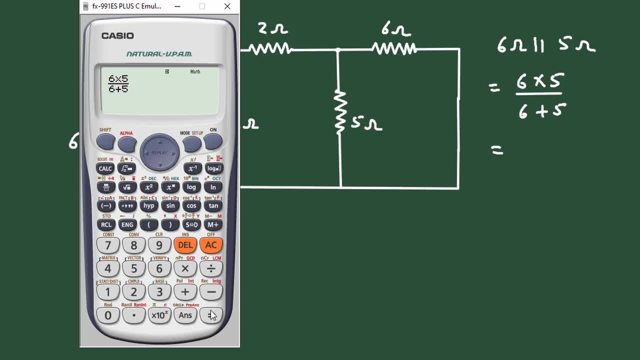 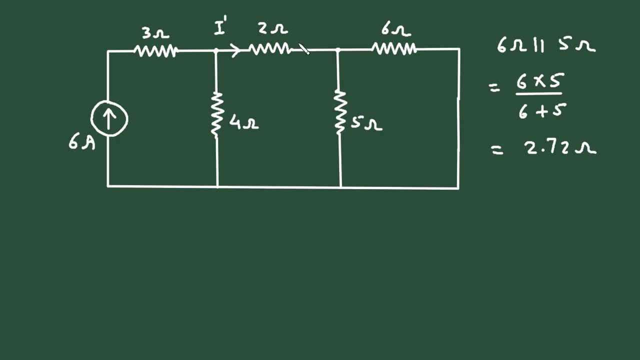 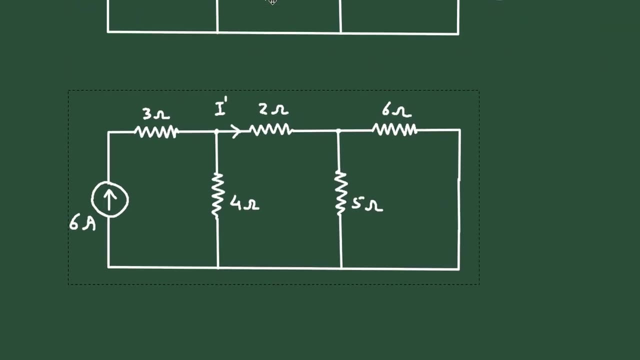 6 into 5, divided by 6 plus 5, so it is 2.72, 2.72 ohm. again, we can copy this circuit. now we can make a single resistor of 2.72 ohm, 2.72 ohm. 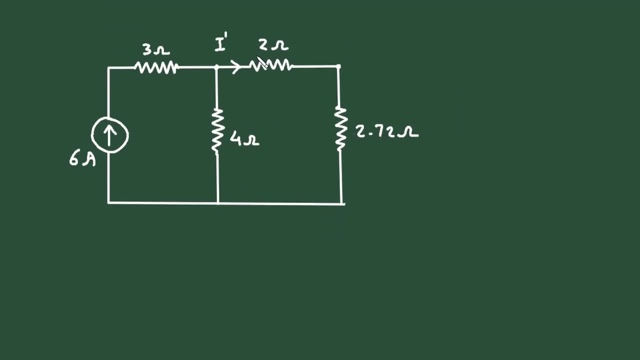 now you can easily find the current through this 2 ohm by using current division rule. so by using current division rule we can find value of I primeI prime will be equal to. here we can write: I prime is equal to this current, that is, 6 ampere multiplied by. opposite branch relationship plus long current, We have seen that we have 2 ohms by mezze circuit. that is the number of transmitters. So here we can write it as 2 ohm Kita over I. next we have to calculate. now we can define. 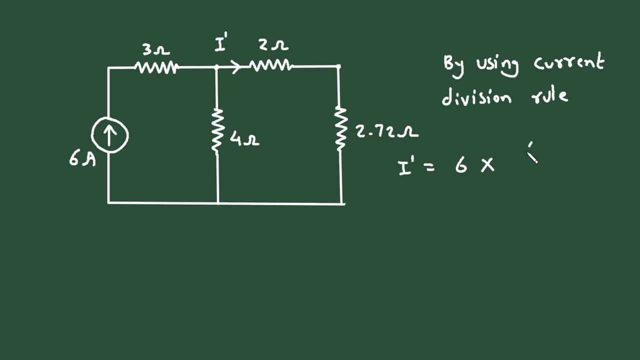 us, as it is 2 boost divided by this 1 resp Inner voltage, which is American Pt U 0 I, is more than 1 best classic temperature. From this material we can write the new profile, the 1st, i realize, resistance. the opposite branch to this is 4 ohm divided by 4 plus 2 plus 2.72.. Now if 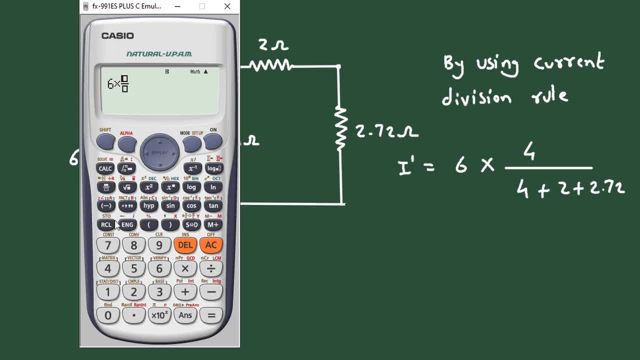 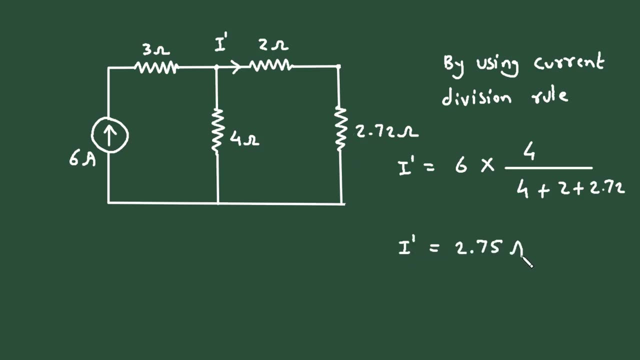 we solve this, so we get 6 multiplied by 4, divided by 4 plus 2 plus 2.72.. So it is 2.75. I prime is equal to 2.75 ampere and the direction is rightward. Now, next we will find the current. 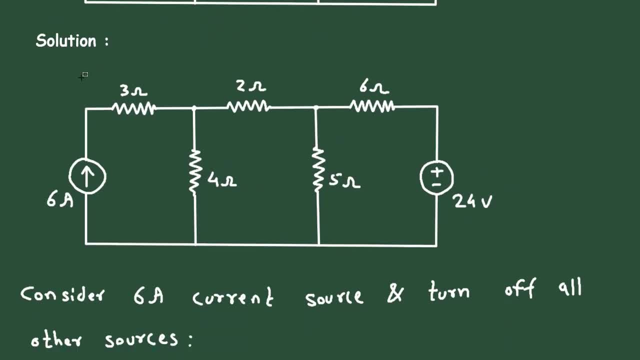 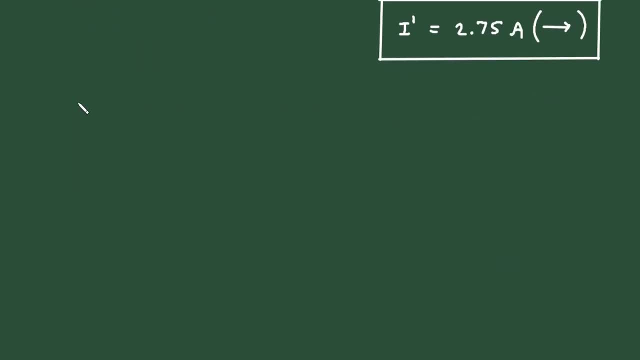 caused by this 24 volt voltage source and that will be our I double prime. So second step is to consider consider 24 volt voltage source and turn off all other sources. turn off all other sources Now. when we turn off this current source, that time this will be open circuit. Now, when this will. 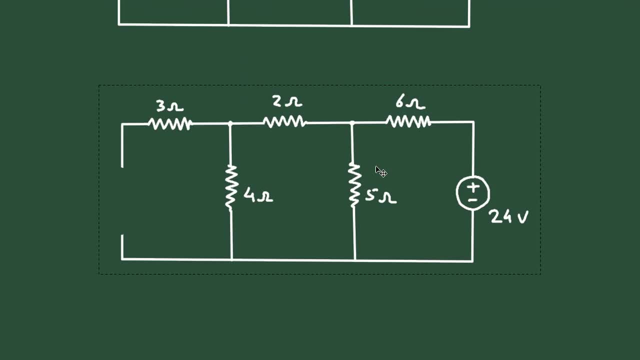 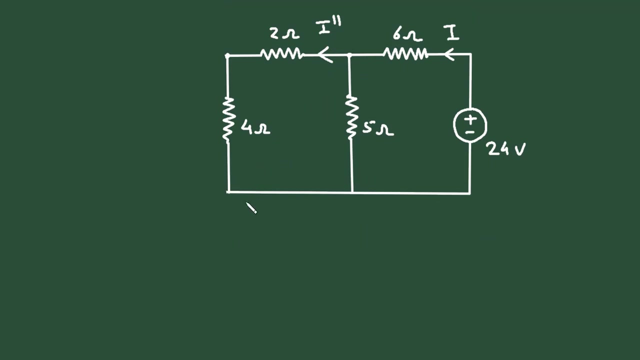 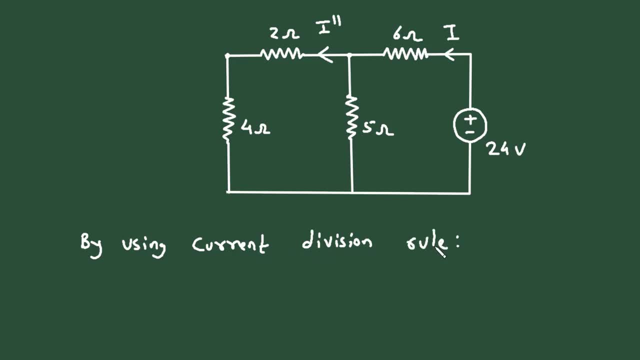 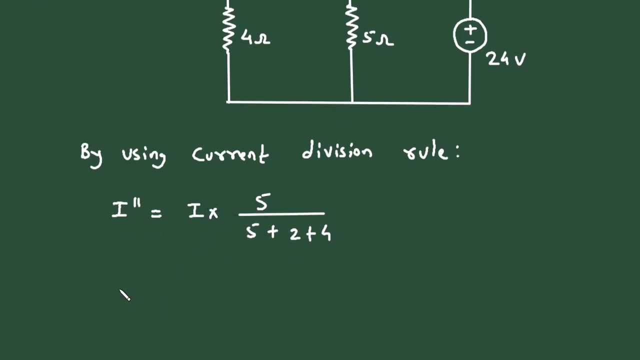 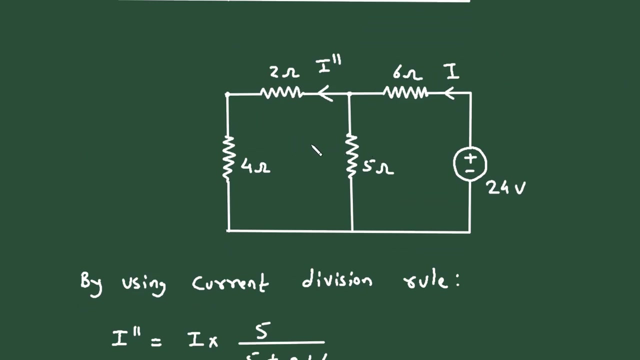 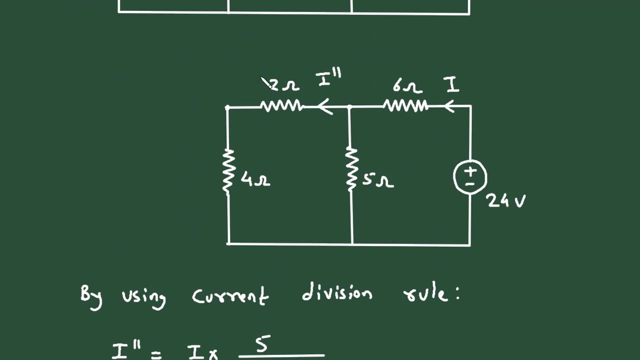 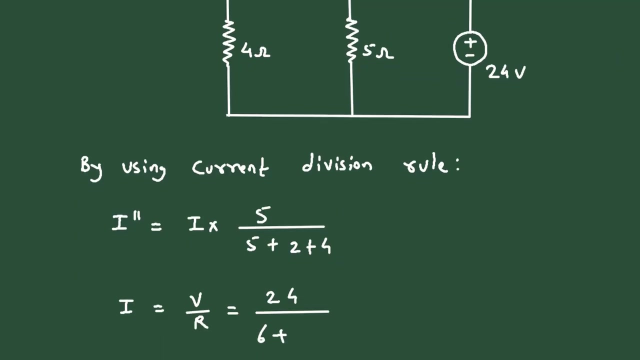 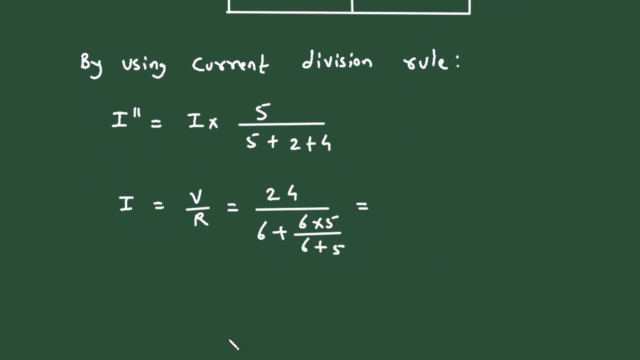 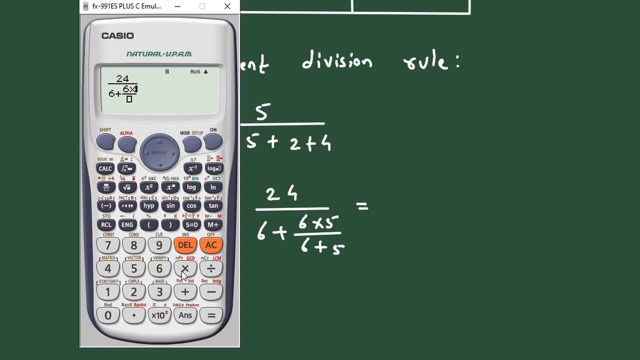 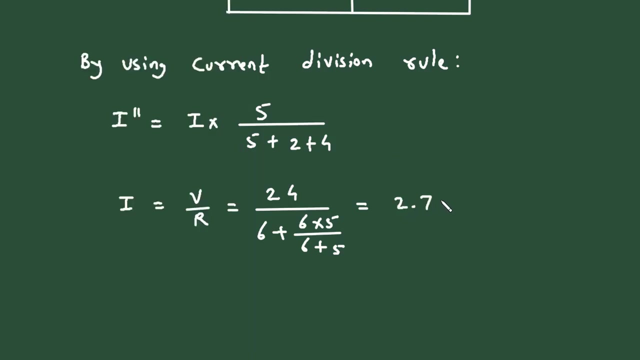 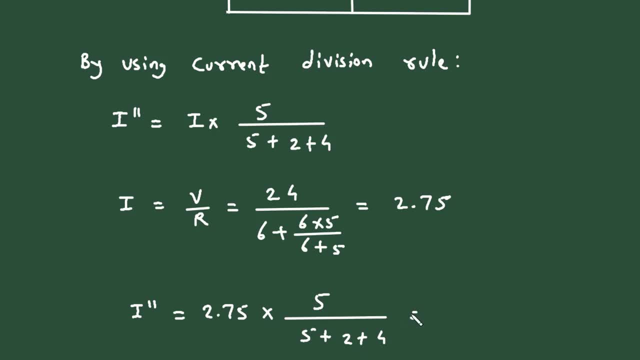 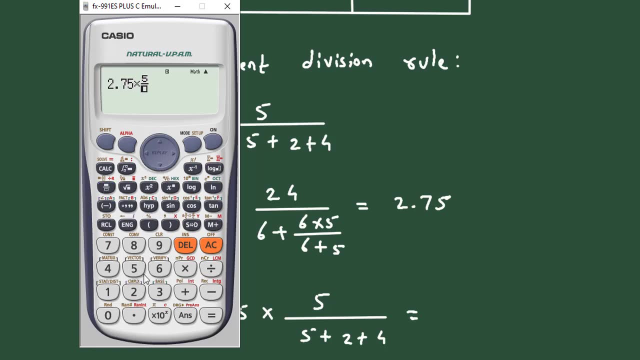 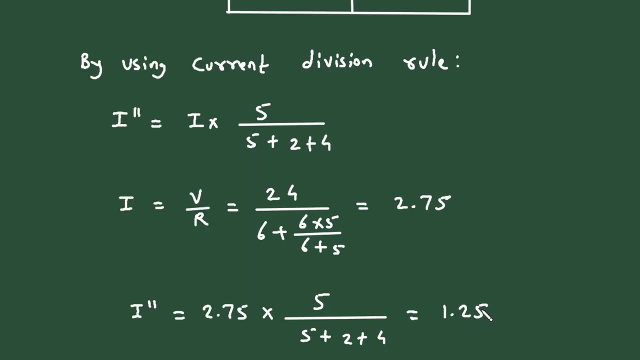 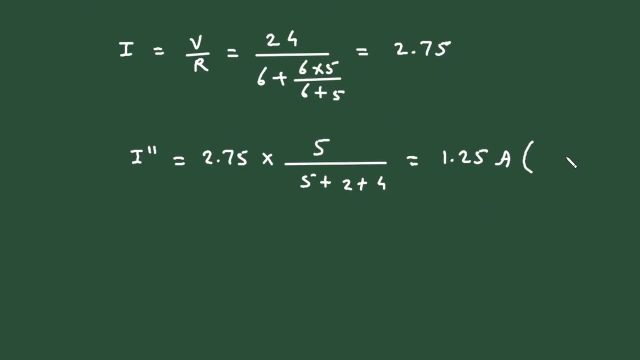 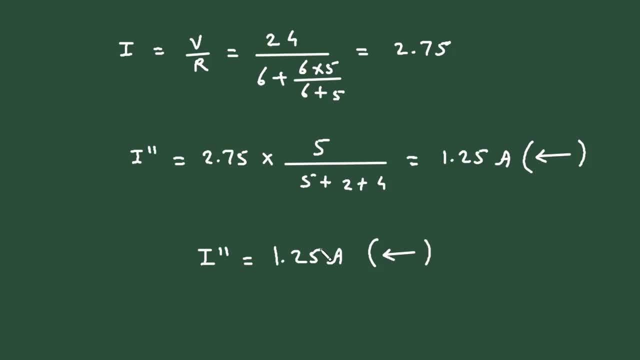 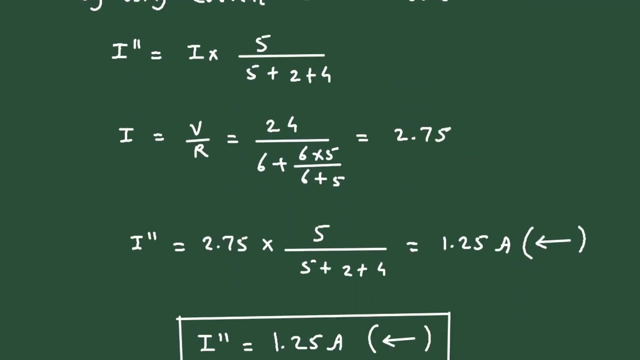 25 ampere and it is leftward. now we can easily find the value of current i, so the current i will be the combination of both i prime and i double prime. here we can see the i prime is rightward and i double prime is leftward. that means we have to subtract.